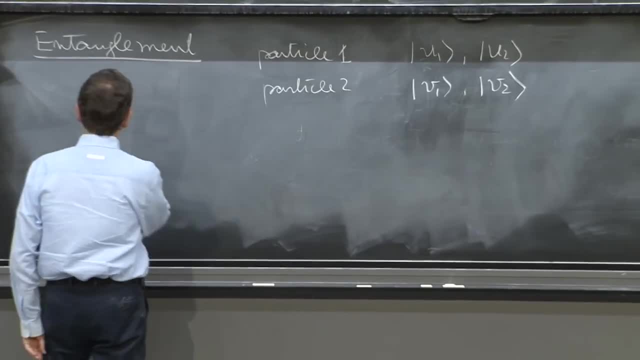 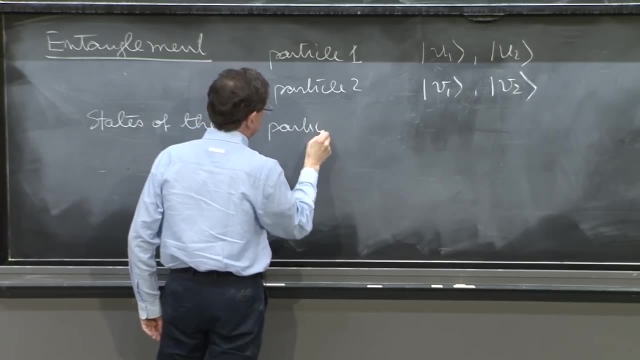 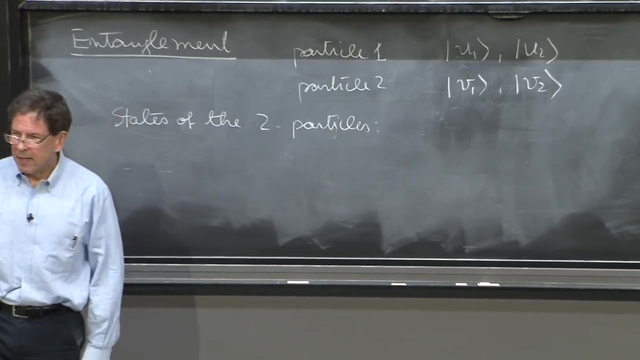 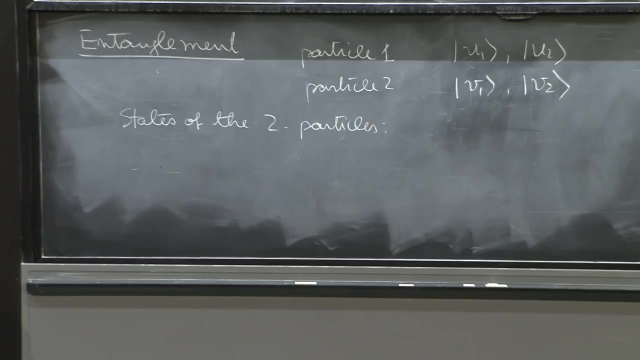 of the two particles. States of the two particles. Two particles. Well, it seems reasonable that, to describe the state of the two particles, they're not interacting. I should tell you what particle 1 is doing and what particle 2 is doing. 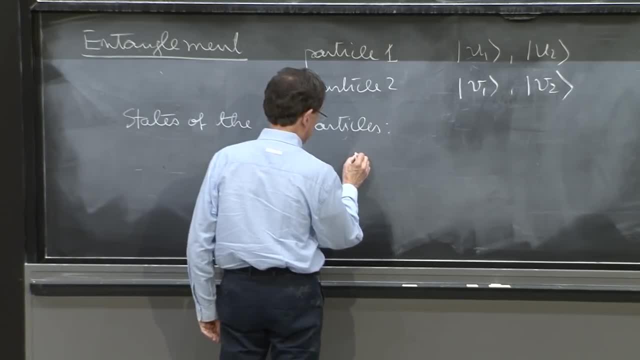 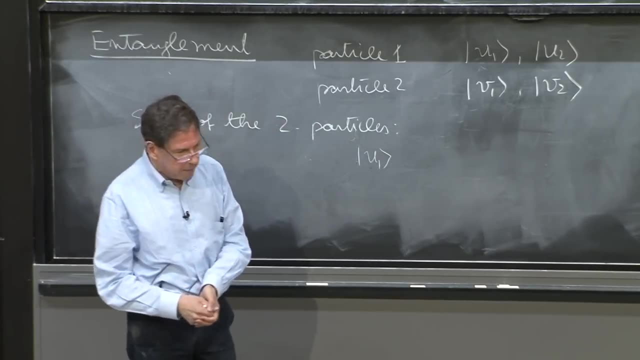 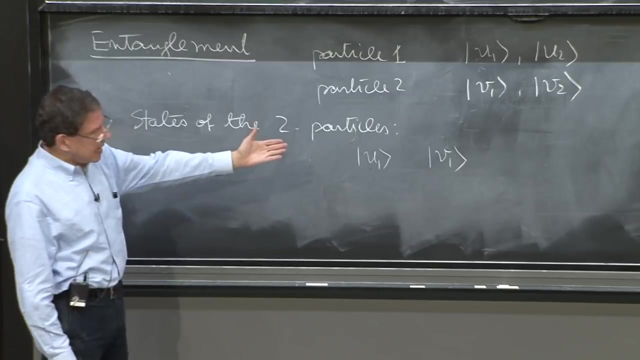 OK, so particle 1 could be doing this, could be u1. And particle 2 could be doing v1.. And in a sense, by telling you that we said what everything is doing, Particle 1 is doing u1.. 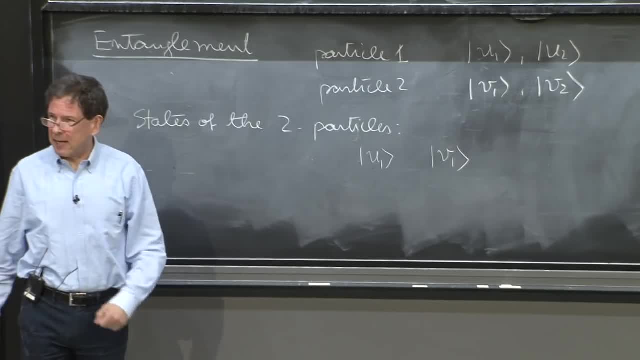 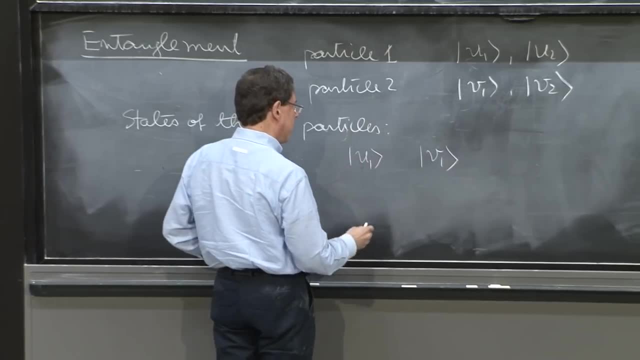 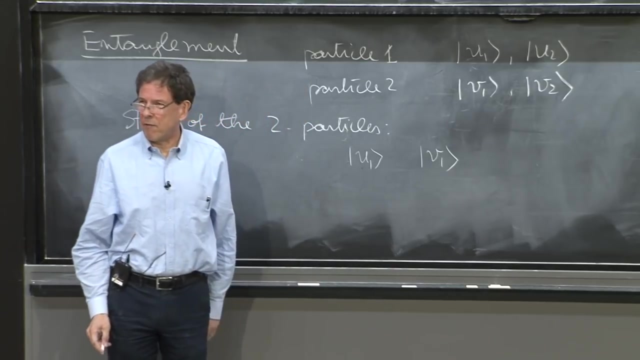 Particle 2 is doing u2.. And mathematically we like to make this look like a state and we want to write it in a coherent way And we sort of multiply these two things. but we must say sort of multiply. 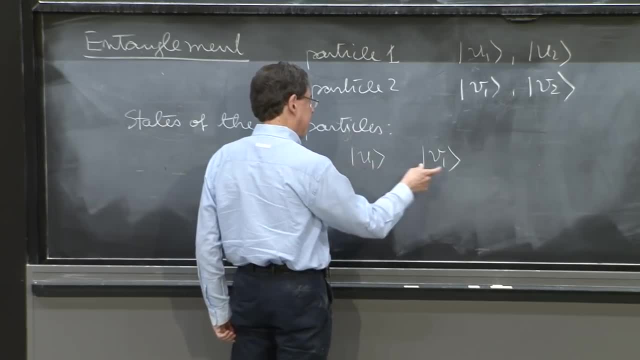 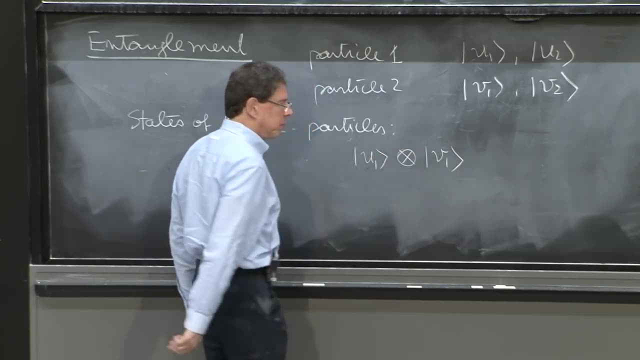 Because it's a strange multiplication. This, you know. we think of them as vectors or states. So how do you multiply states? So you put something called the tensor product, a little multiplication like this, So you could say: don't worry. 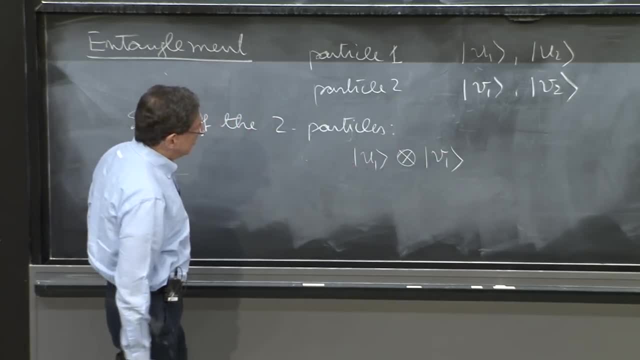 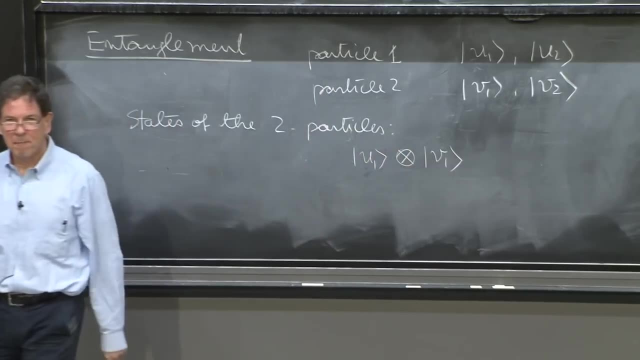 It's kind of like a product, And it's the way we do it. We don't move things across. We list the first state here, the second state here, And that's a possible state. Now I could have a different state. 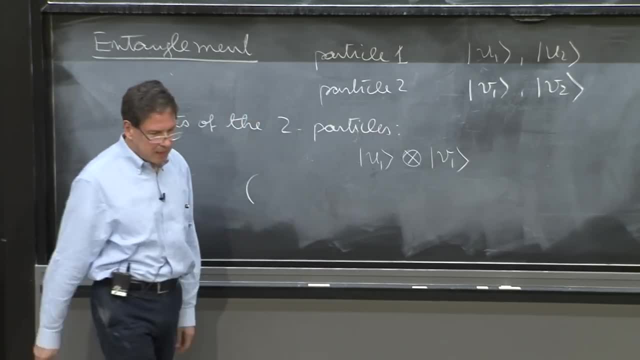 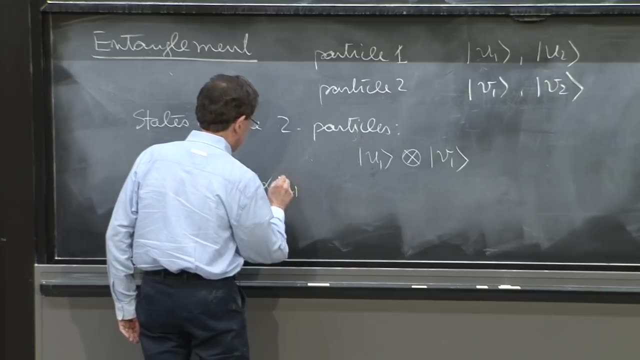 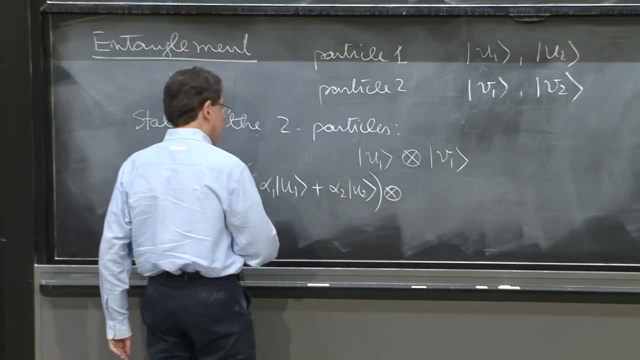 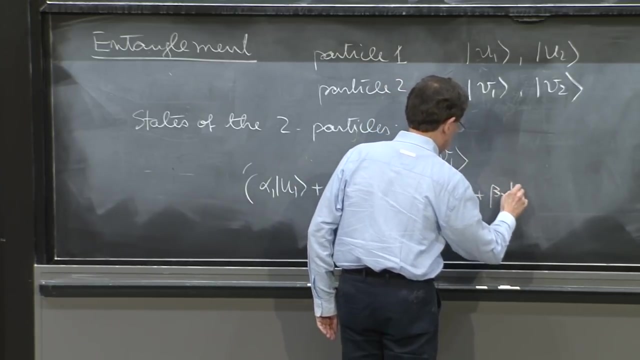 Because particle 1,, in fact, could be doing something a little different. Could be doing alpha 1 u1 plus alpha 2 u2.. And maybe particle 2 is doing something like doing beta 1 v1 plus beta 2 v2.. 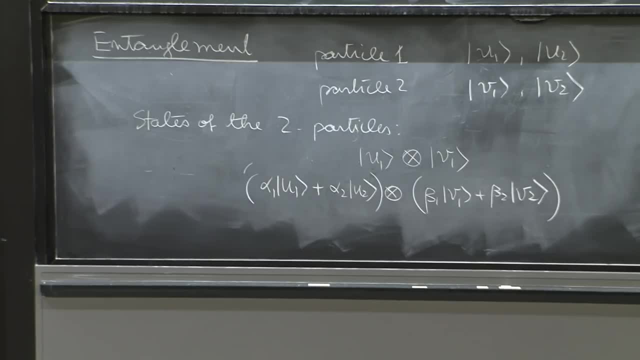 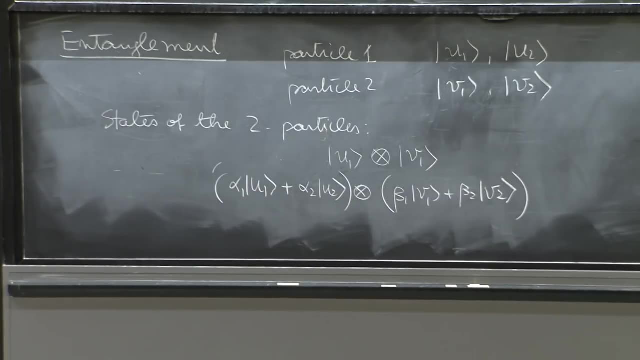 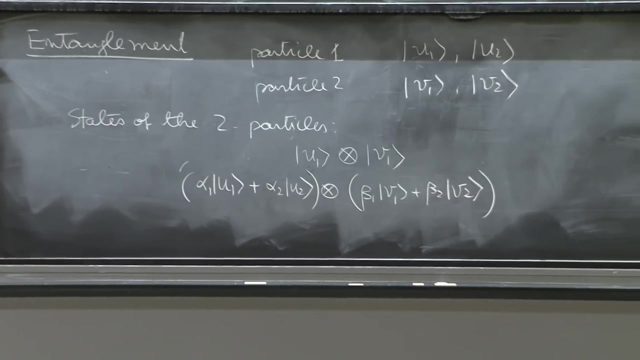 And this would be all right. I'm telling you what particle 1 is doing And I'm telling you what particle 2 is doing. And the rules of tensor multiplication or this kind of multiplication to combine those states are just like a product, except that, as I said, you never 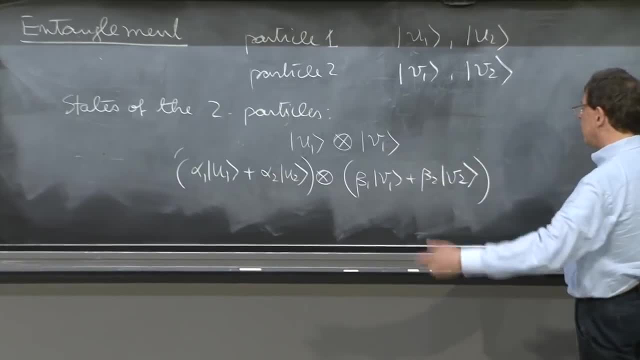 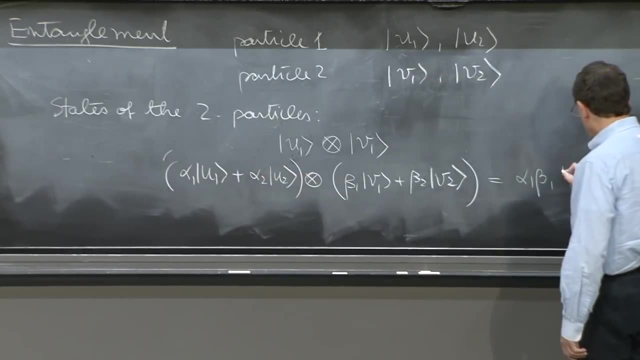 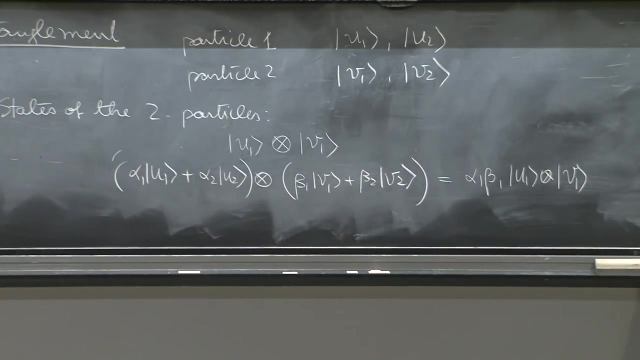 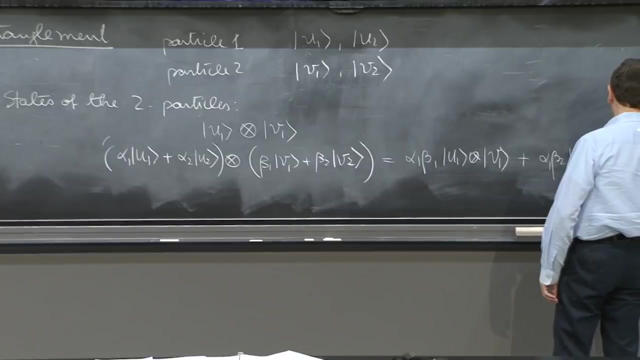 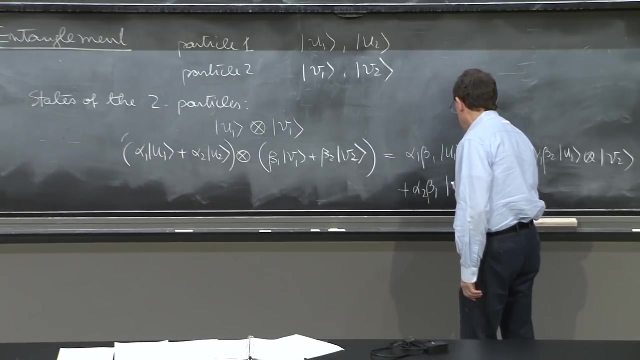 the states across. So you just distribute. So you have alpha 1- beta 1.. The number goes out: u1- v1.. That's the first factor. Plus alpha 1- beta 2: u1- v2.. Plus alpha 2- beta 1: u2- v1.. 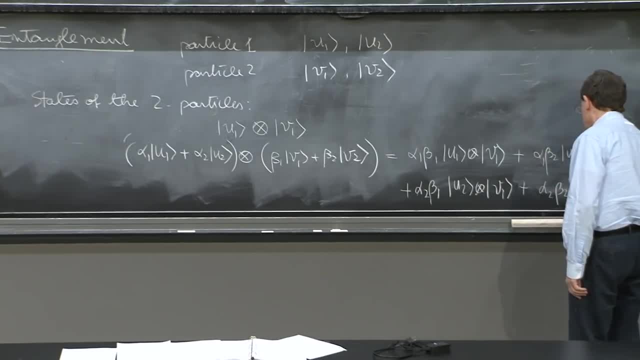 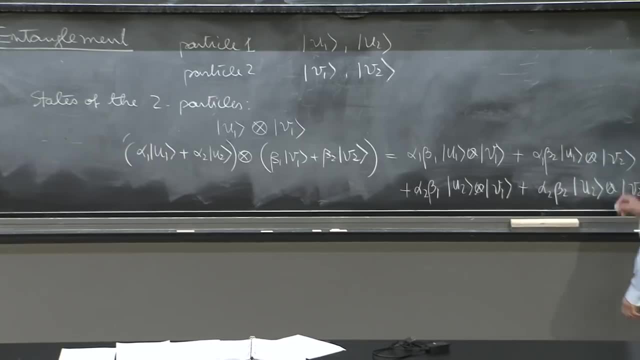 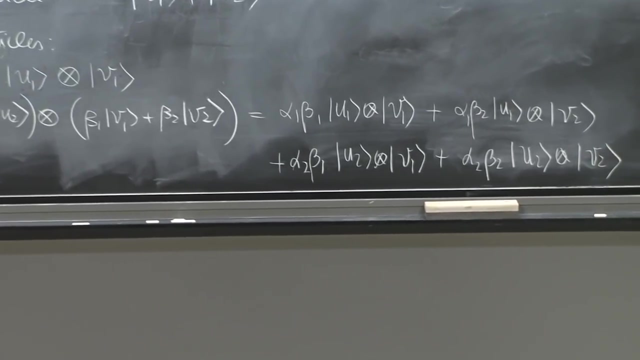 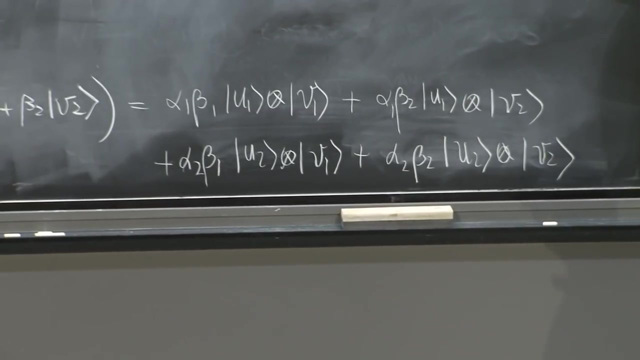 Plus alpha 2, beta 2, u2, v2.. I think I got it right. Let me know, I just multiplied and got the numbers out. The numbers can be moved out across this product. OK, so that's a state And that's a superposition of states. 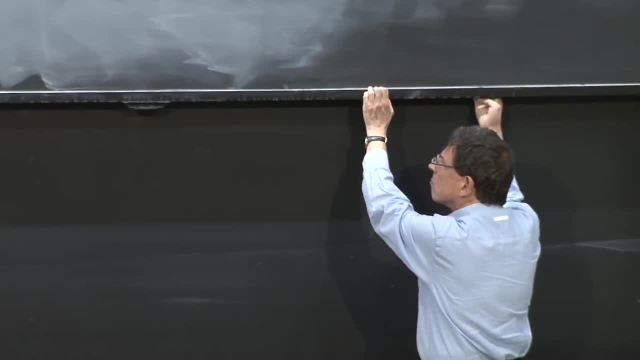 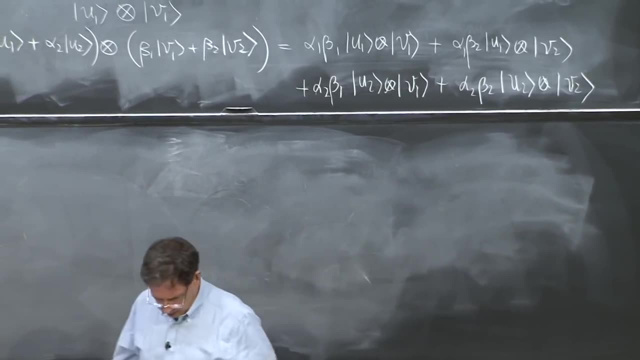 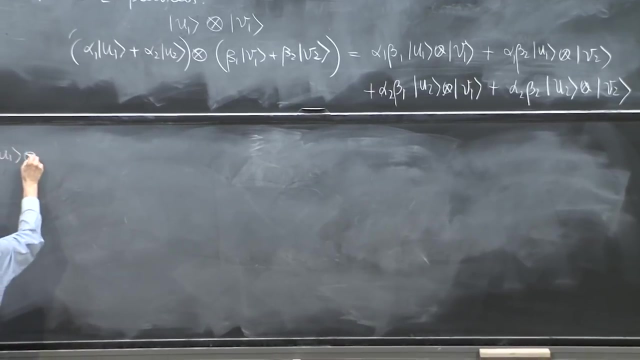 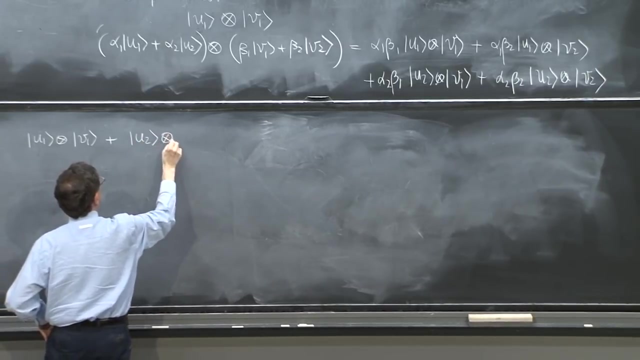 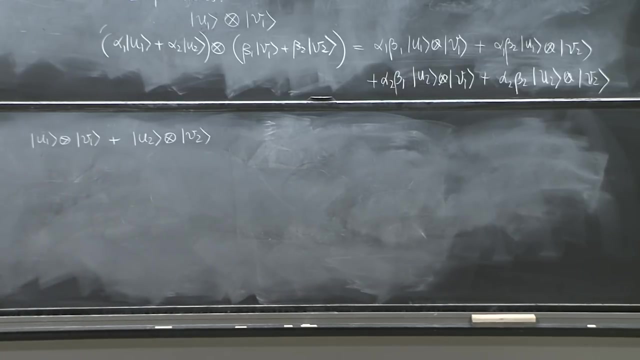 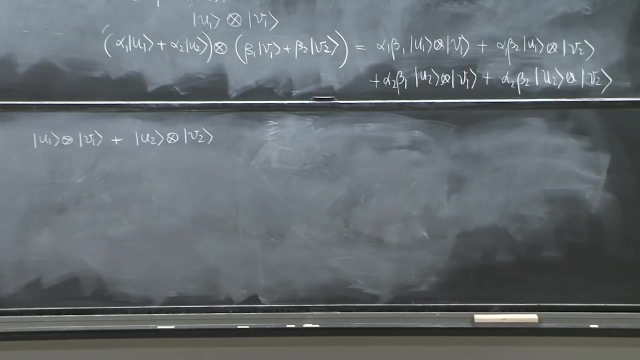 So actually I could try to write a different state. now, You see, we're just experimenting, But here is another state: u1 v1.. u1 v1 plus u2 v2.. Now this is a state that actually seems different. 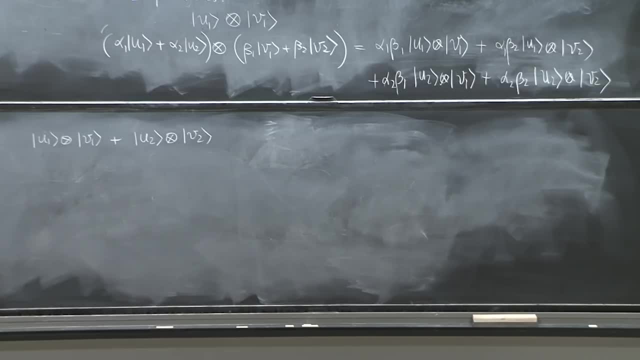 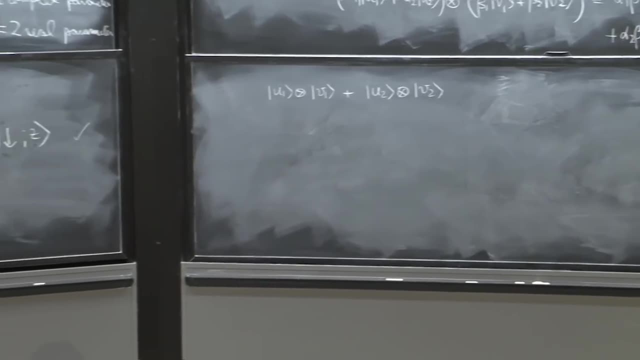 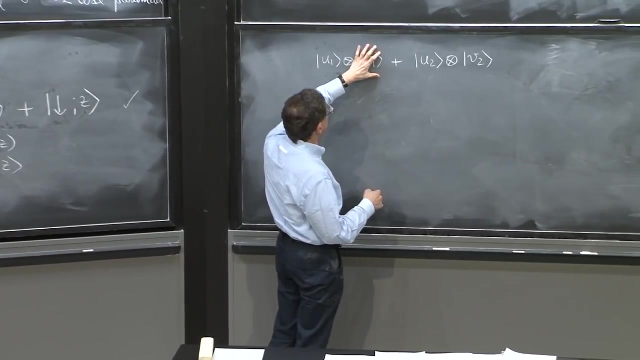 Why different? Because I don't seem to be able to say that what particle 1 is doing And what particle 2 is doing Separately. You see, I can say when particle 1 is doing u1, particle 2 is doing v1.. 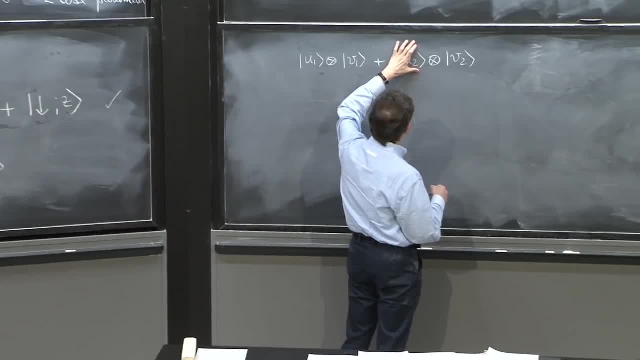 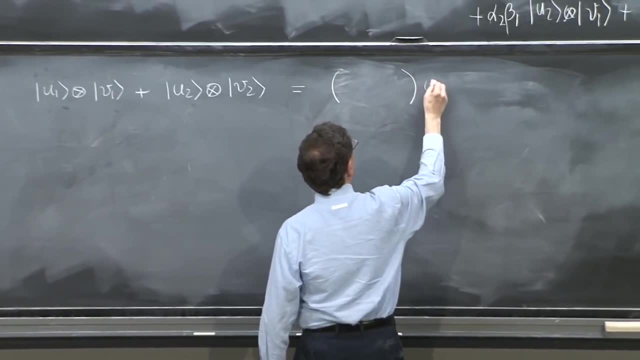 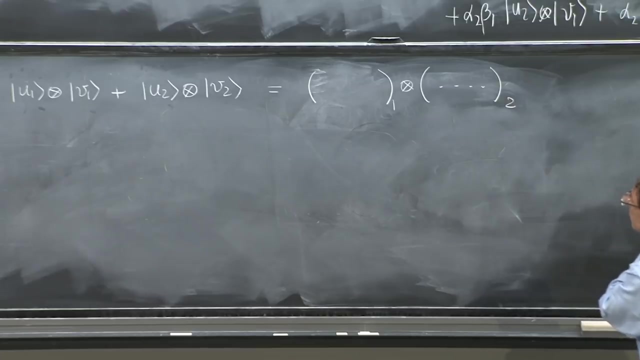 And when particle 2, 1 is doing u2, this is v2.. But can I write this as some state of the first particle times some state of the second particle? Well, let's see, Maybe I can, And I can write it in this form. 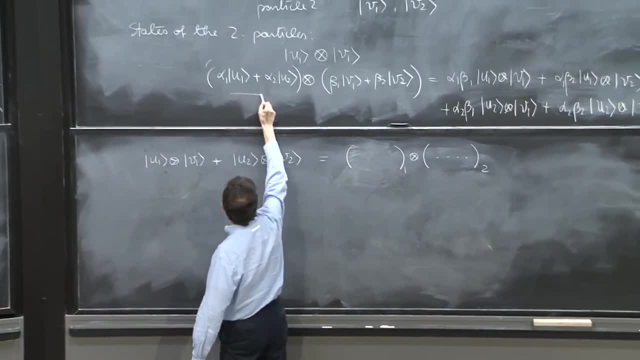 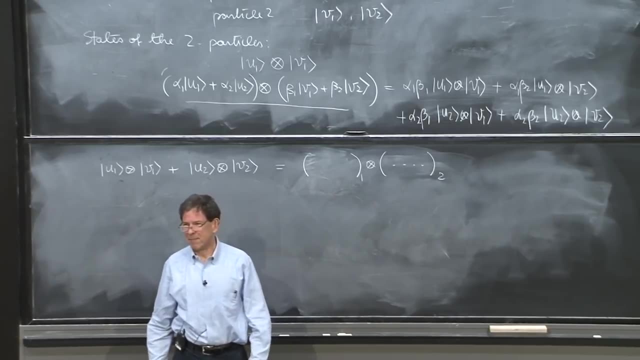 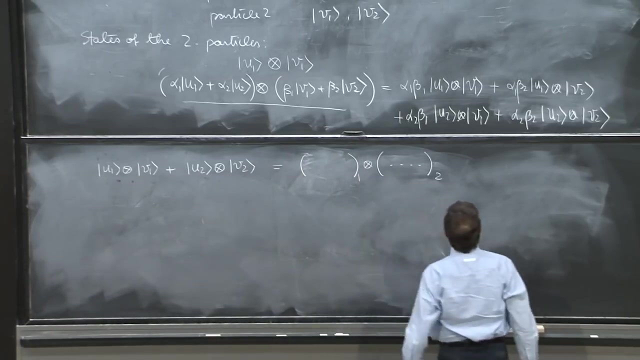 This is the most general state that you can say: Particle 1 is doing this And particle 2 is doing that. So can I do that? Well, I can compare these two terms with those And I conclude that alpha 1, beta 1 must be 1.. 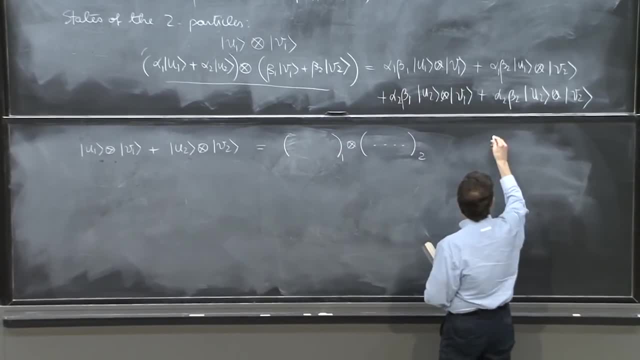 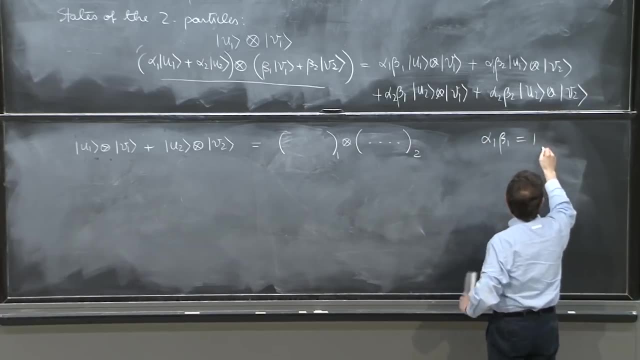 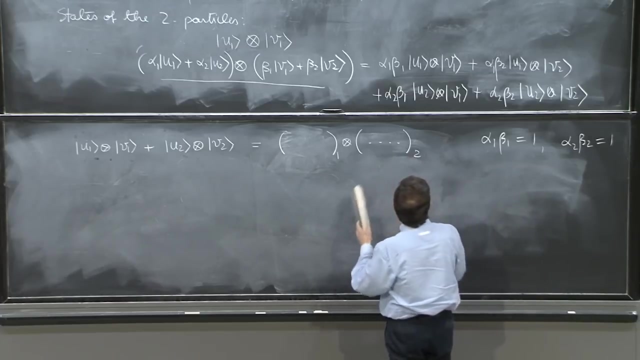 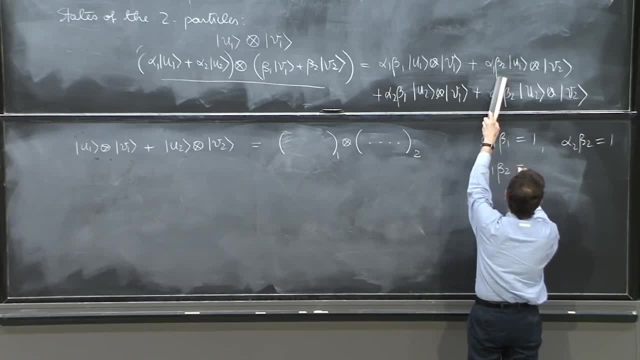 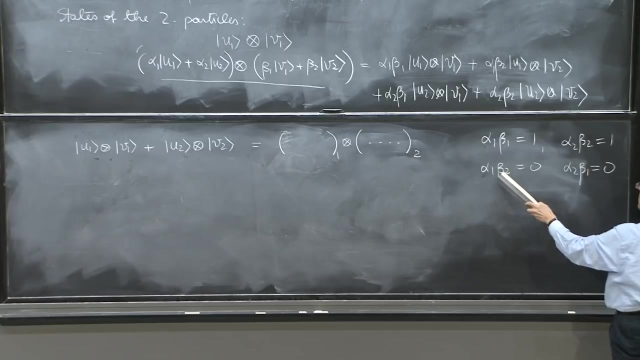 So alpha 1- beta 2 must be 0. And alpha 2- beta 1 must be 0. And that's a problem, Because either alpha 1 is 0.. 0, which is inconsistent, or beta 2 is 0,. 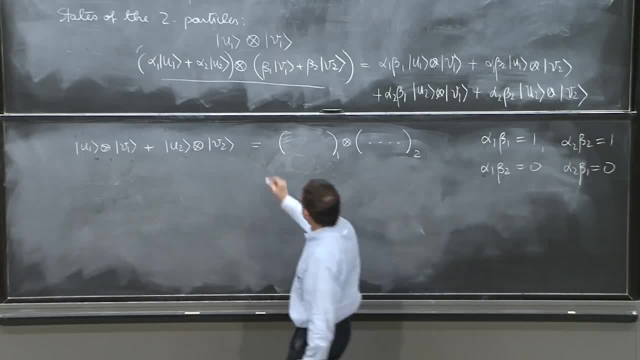 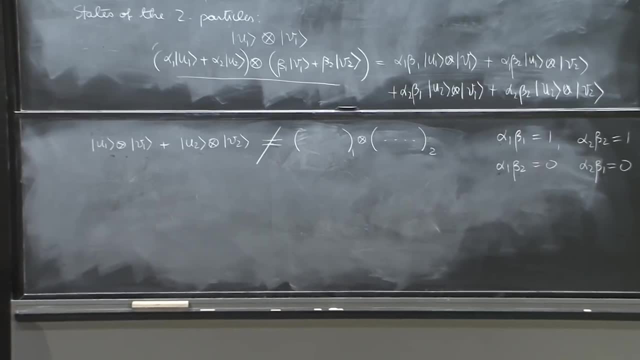 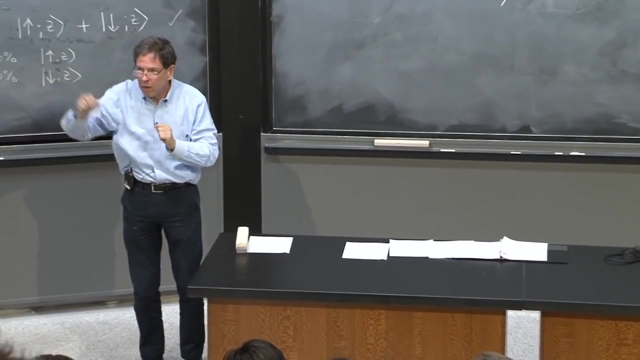 which is inconsistent with that. So no, this state is unfactorizable. It's a funny state in which you cannot say that this quantum state can be described by telling what the first particle is doing and what the second particle is doing. What the first particle is doing depends on the second. 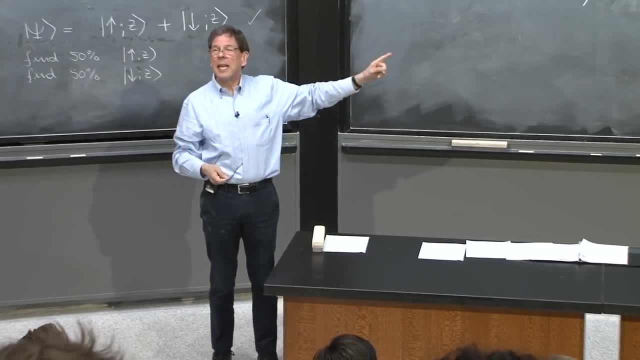 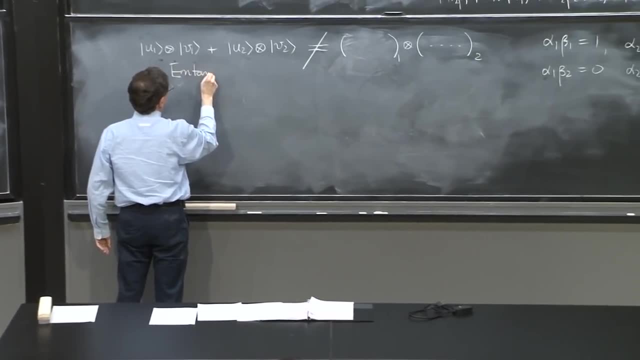 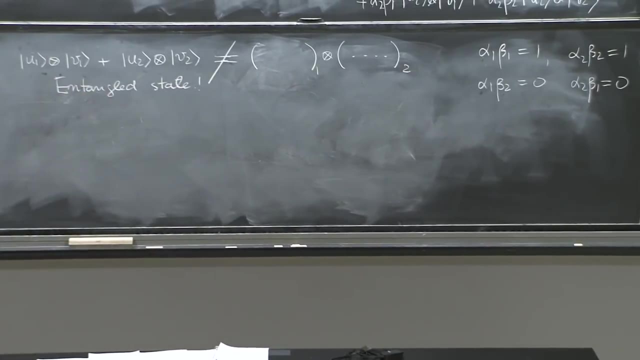 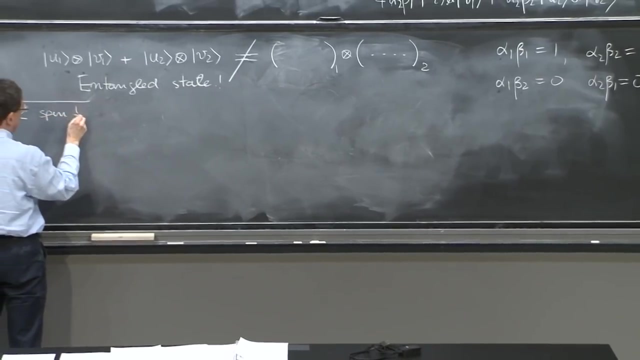 and what the second is doing depends on the first. This is an entangled state, And then we can build entangled states in our very strange states, So with two particles with space, So with two spins. for example, we can build an entangled states of two spin 1 half particles. 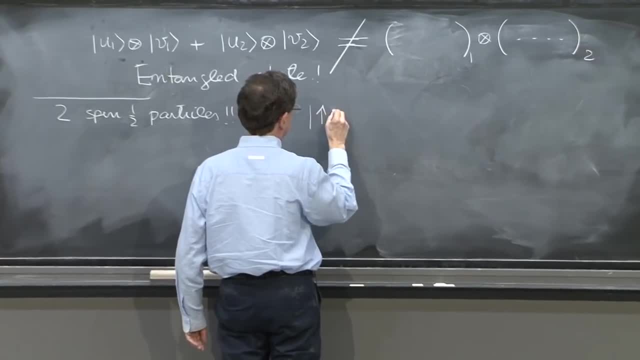 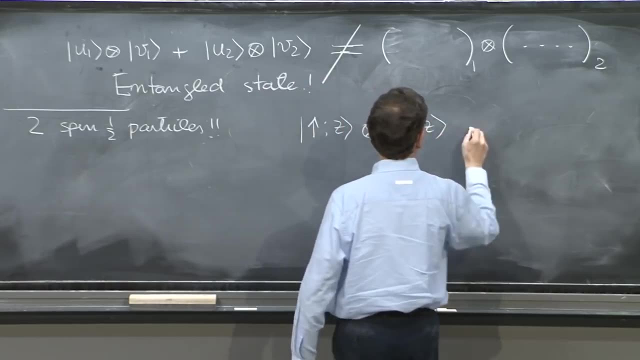 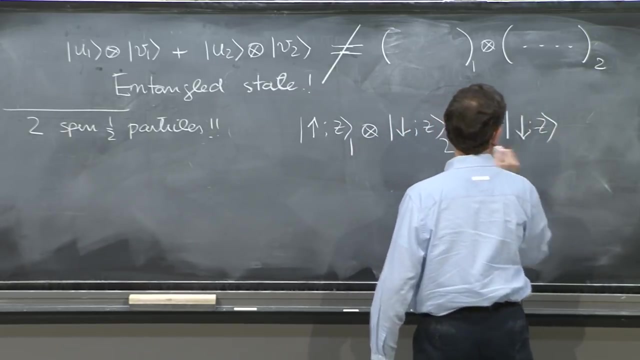 And this state could look like this: The first particle is up along z and the second particle is down along z, plus A particle, And the second particle is down along z for the first particle, But the second is up along z. 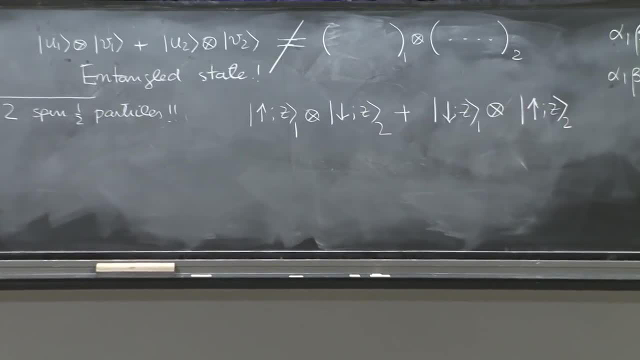 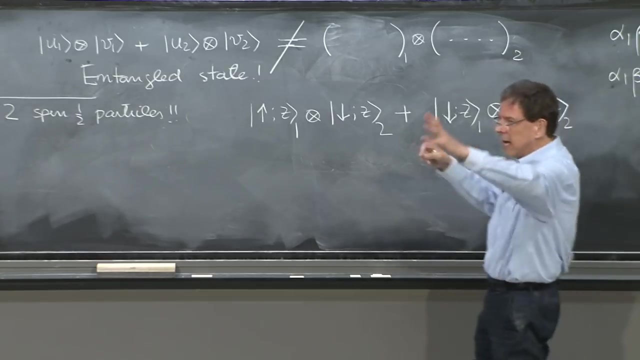 And these are two spin 1 half particles And in the usual notation these experiments in quantum mechanics, in black hole physics, people speak of Alice and Bob. Alice has one particle, Bob has the other particle. Maybe Alice is in the moon and has her electron. 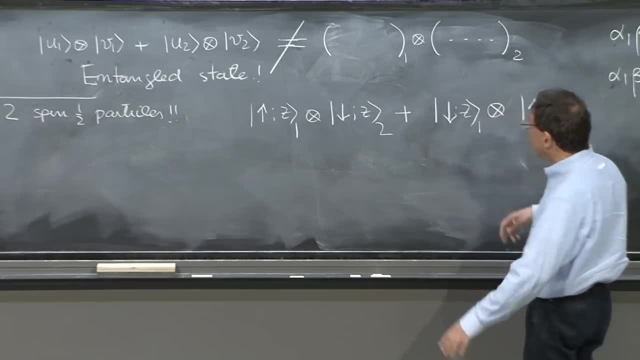 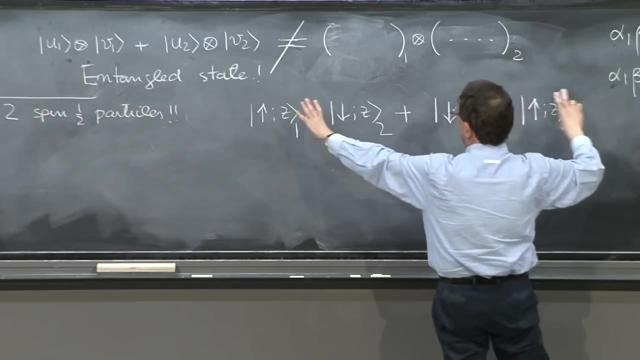 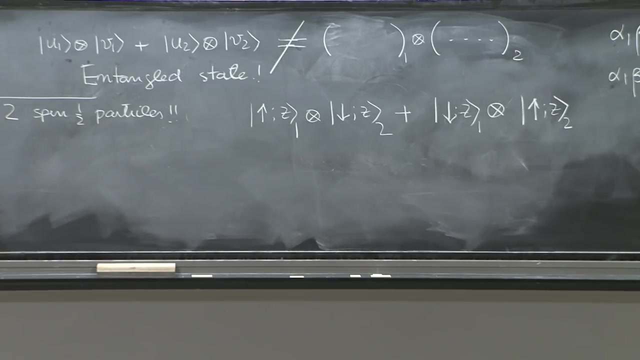 And Bob is on Earth and has his electron, And the two electrons, one in the Earth and in the moon, are in this state. So then we say that Alice and Bob share an entangled pair And all kinds of strange things happen. People can do those things in the lab- Not quite. One can do it, One in the Earth and one in the moon, But one photon at one place and another photon entangled with it at 100 kilometers away. That's pretty doable. 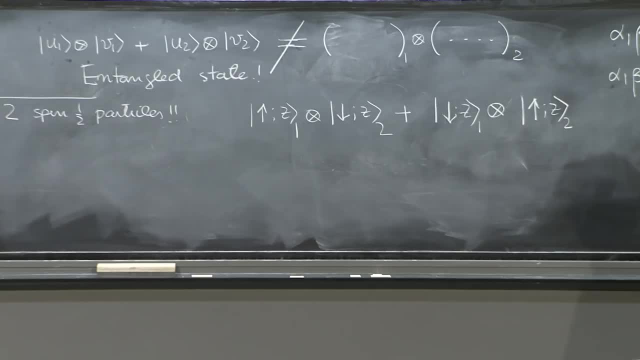 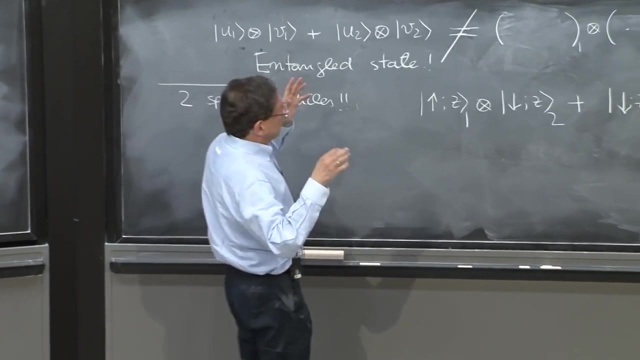 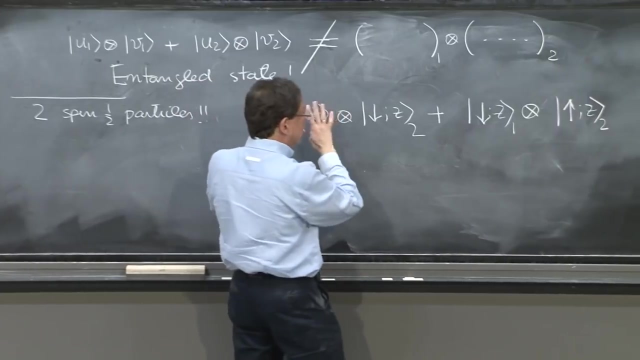 And they are in this funny state in which their properties are correlated in surprising ways. So what happens here? Suppose Alice goes, or let's say Bob Goes, along and measures his spin And he finds his spin down. So you look here. 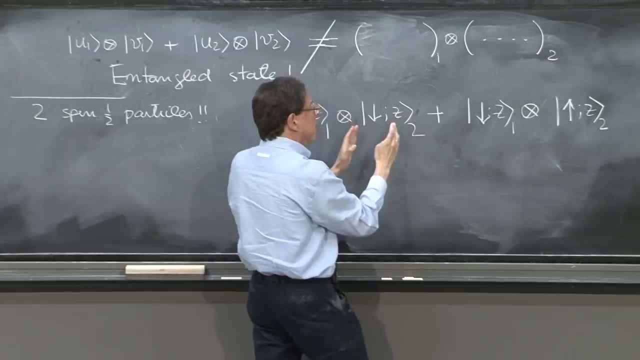 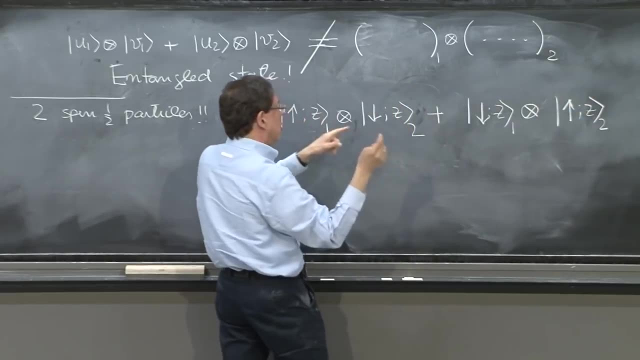 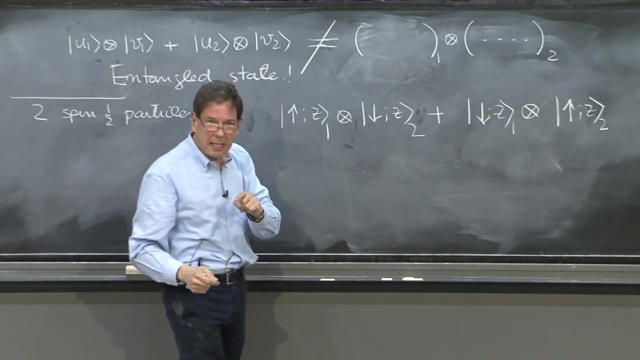 Oh, here is down for Bob. So at this moment the whole state collapses into this, Because up with Bob didn't get realized. So once Bob measures and he finds down, the whole state goes into this. So if Alice on the moon or in another galaxy, 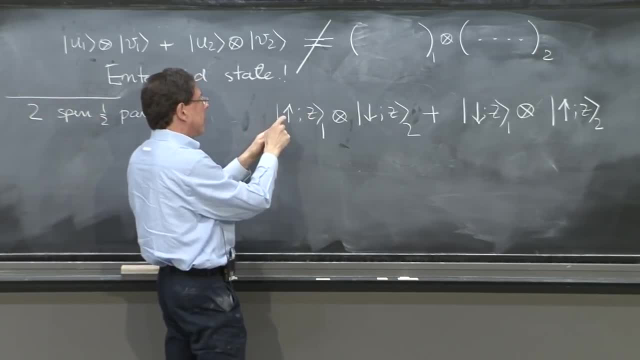 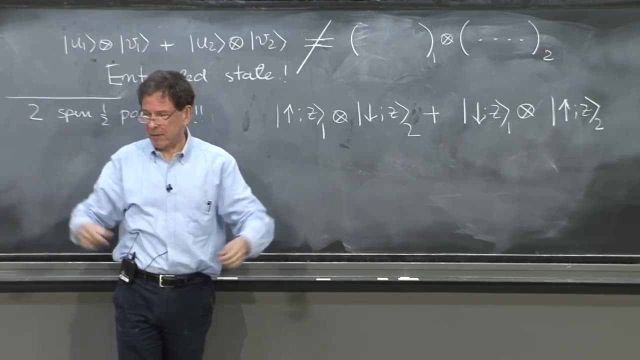 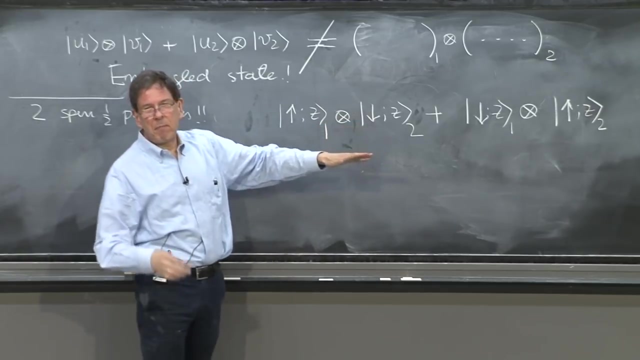 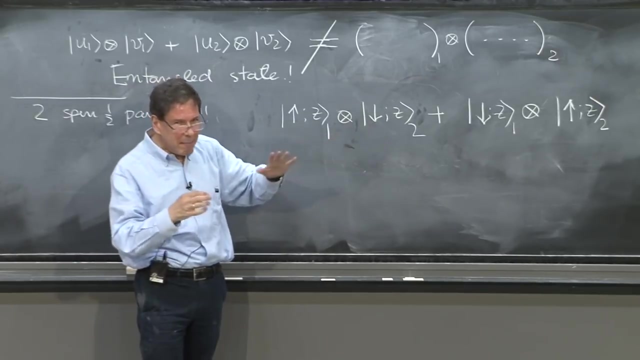 at that instant. looks at her spin. she will find it up Before light. has had time to get there instantaneously it will go into this state. People were sure somehow this violates special relativity. It doesn't You, somehow, when you think about this carefully? 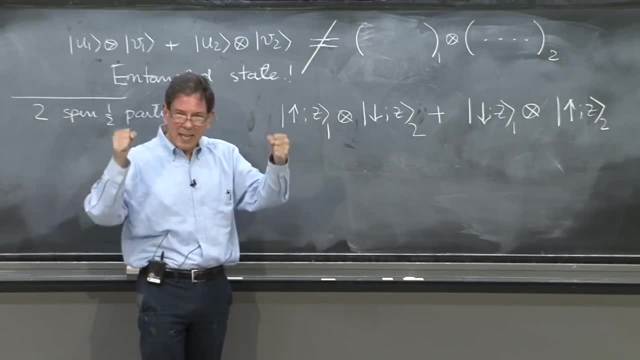 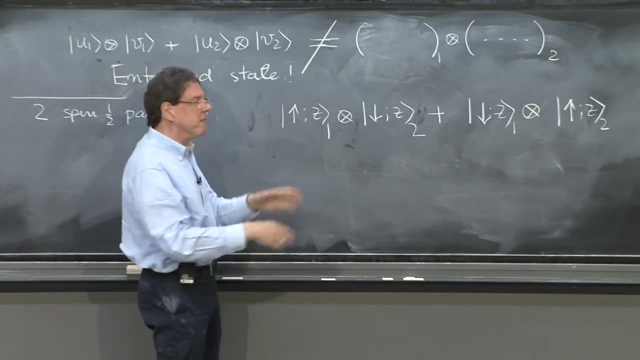 can't quite send information, But it collapses into this state. It collapses instantaneously in quantum mechanics. Somehow Bob and Alice cannot communicate information by sharing this entangled pair. But it's an interesting thing why it cannot happen. Einstein again objected to this. 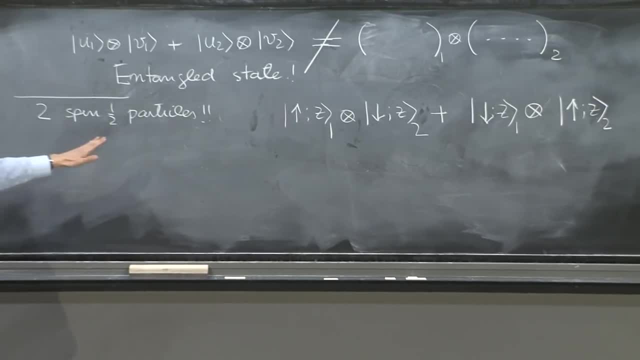 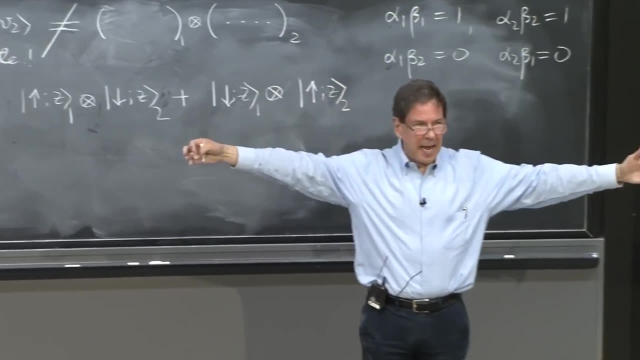 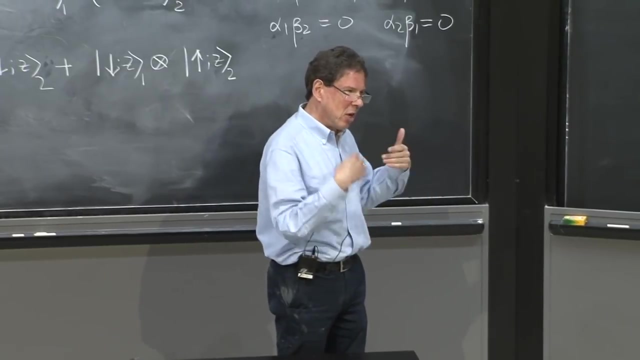 And he said: this is a fake thing. You guys are going to share, And now, of course, they have to share many entangled pairs to do experiments. So maybe 1,000 entangled pairs And Einstein would say: no, that's not what's happening.